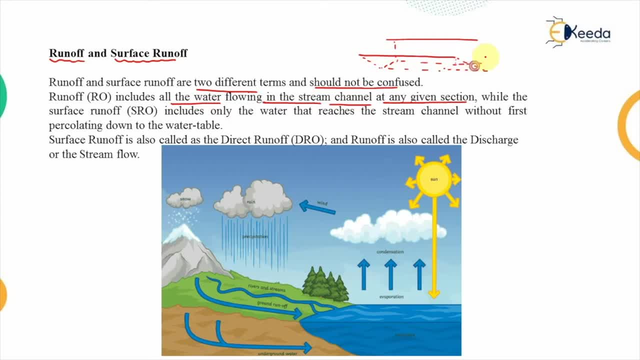 Let's say this is the stream channel which is carrying the water. So the water which will be flowing through this, that is calculated as runoff, While the surface runoff, that includes only the surface runoff, Only that water that reaches the stream channel without first percolating down to the water table. 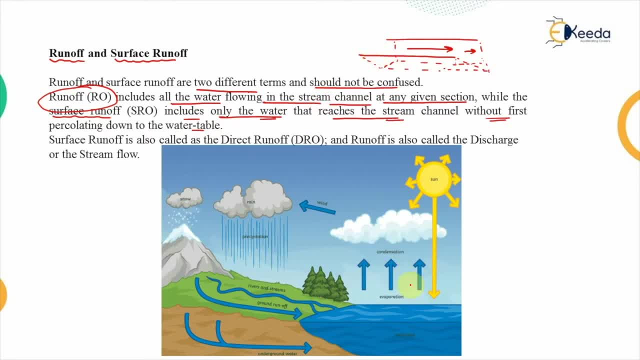 That means this is the typical water cycle which starts, let's say, at the evaporation. So when a certain amount of water it gets heated up because of the constant exposure to the heating bodies, for example the sun, Because of that the certain vapors will be formed. 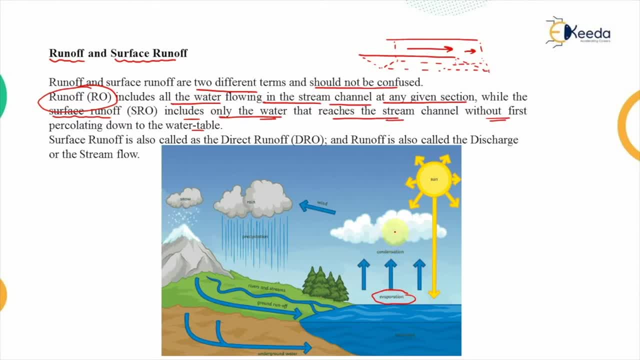 And those vapors, upon condensation, form a cloud Which, upon the effect of the wind that moves towards the land side And when it reaches the sufficient height and the suitable conditions, it drops down in the form of the precipitation. 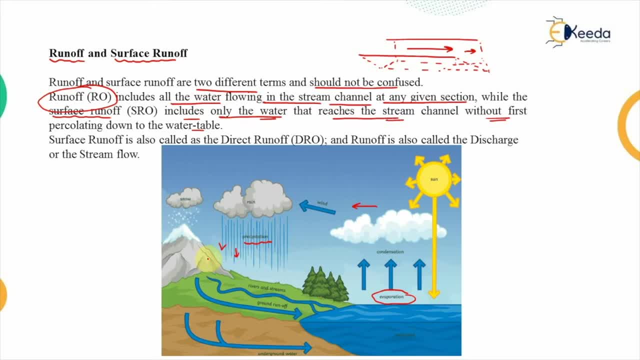 This precipitated water that follows a path on the land surface, This water which is draining or flowing off, And this precipitation which is draining or flowing on the catchment area through a surface channel. That is known as the runoff, In general, the component of the precipitation that has not evaporated nor transpired. 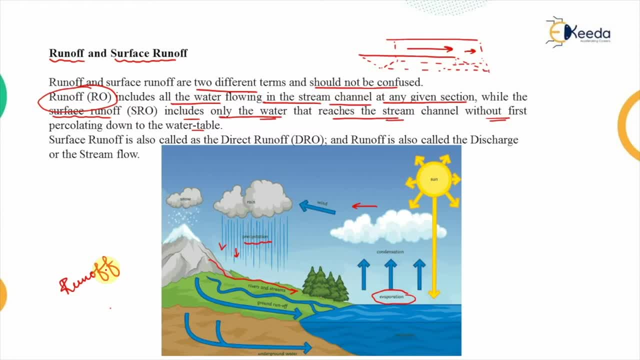 That is known as the runoff And that is the remaining output Of the catchment area per unit time. Now, depending upon the location where this runoff is flowing And finally, where it is meeting the stream, It is classified in different categories. 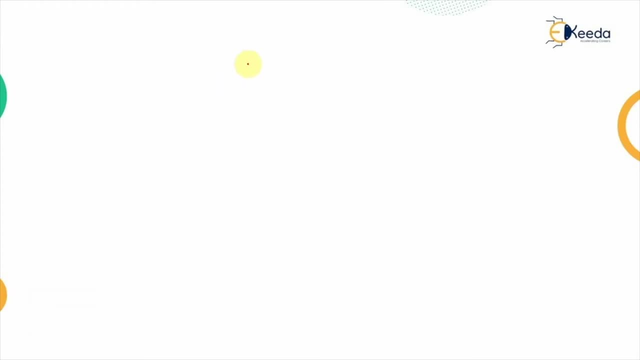 So, depending upon the location of the runoff, This runoff is classified into majorly two categories. The first category, that is known as the surface runoff- The water which is flowing over the catchment area On the surface streams, That is surface runoff. 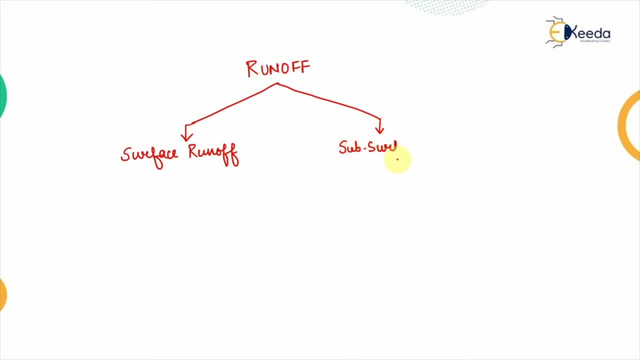 If it is flowing below the earth surface. That is known as the subsurface runoff. Now, this subsurface runoff, That is further classified into two different categories, That is, If within the earth, If the water is flowing on the top layer. 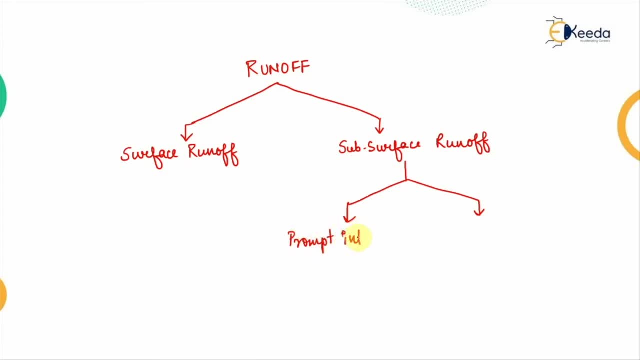 That means within the crust of the earth surface. If the water is flowing, Then that is known as the prompt interflow, Which is also known as the seepage water, And the water which percolates down to the deeper depths, That is known as the delayed flow. 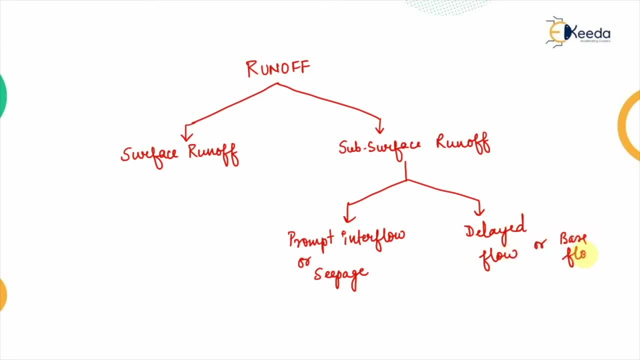 Or that is also known as the Base flow. So, depending upon the location of the runoff, This is the classification of the runoff- And it also depends upon the location Where the runoff is finally meeting the stream. So, as you can see in this image, 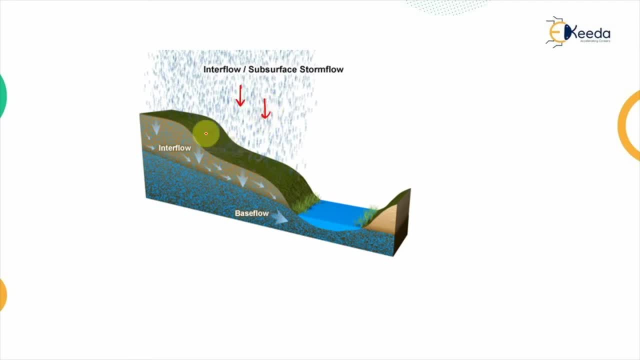 When the precipitation is happening. Depending upon the topography of the area, Certain amount of the water Which has precipitated, It directly joins the stream And it gets collected in the depressions, If there is any. The remaining amount, It gets seeping down into the ground. 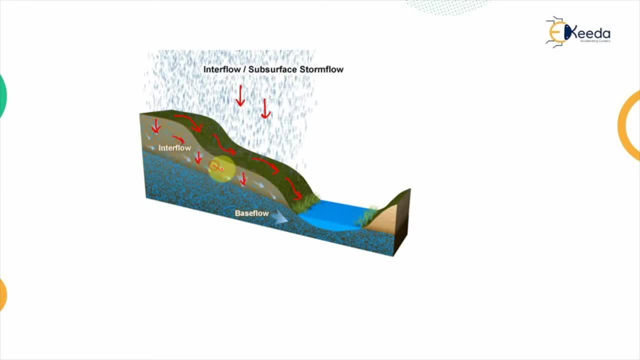 And flows laterally And that moves under the earth surface, So that is known as the interflow, And the rest of the amount Which percolates at the deeper depths And then flows parallelly, That is known as the base flow. 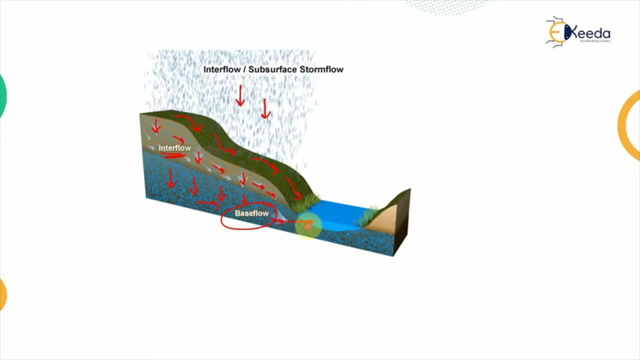 Now, this base flow That may contribute immediately to the collection area Or may not. That depends upon the depth of the base flow. So this first one, That is the surface runoff, That is the first type of the runoff. So when a precipitation occurs, 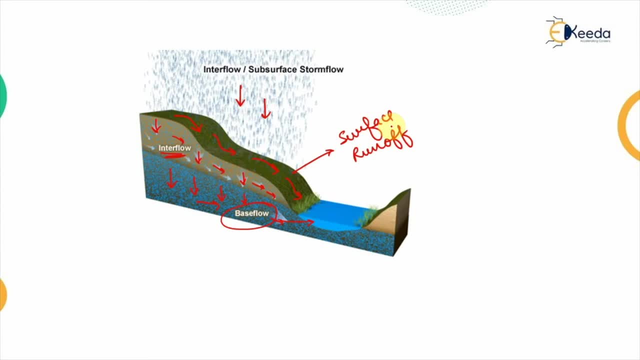 Over a catchment area, It will first fulfill the requirement of the evaporation That is required for the hydrological cycle to continue or sustain, Then the transpiration needs of the plants, Then if there are any depression storages, For example if there is certain area. 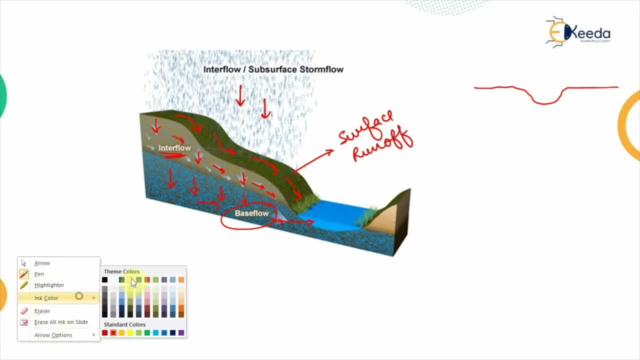 In which this depression is made. So the water, when it will be flowing, It will be getting collected in this depression storage, And once it is completely filled, Only then the runoff will be moving right. So, after fulfilling all of these needs, 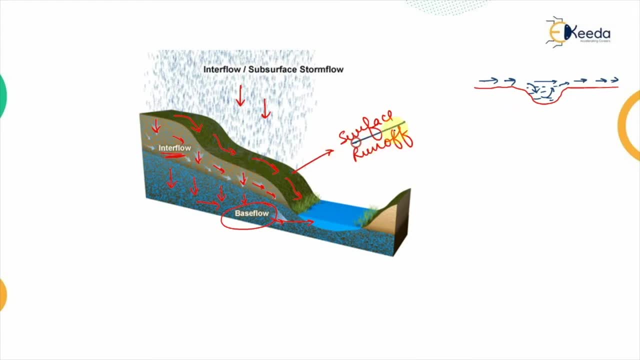 The water which is still flowing over the surface. That is known as the surface runoff. Now, usually all the time, This water flows over the land- Therefore, this is also known as the over land flow- And it reaches the catchment outlet. 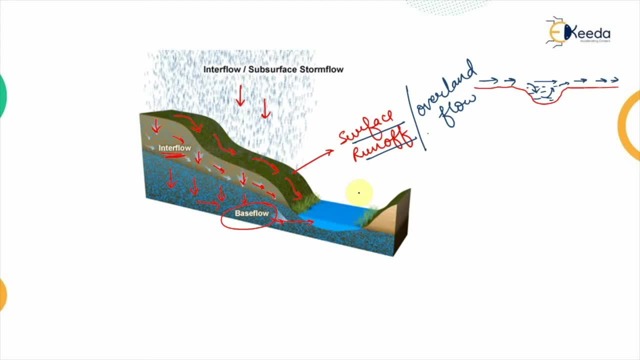 And is termed as the surface runoff. Now the second category of the runoff That is below the earth surface And that is known as the subsurface runoff. Now this is further classified into two categories: The prompt interflow, Which is the part of the precipitation. 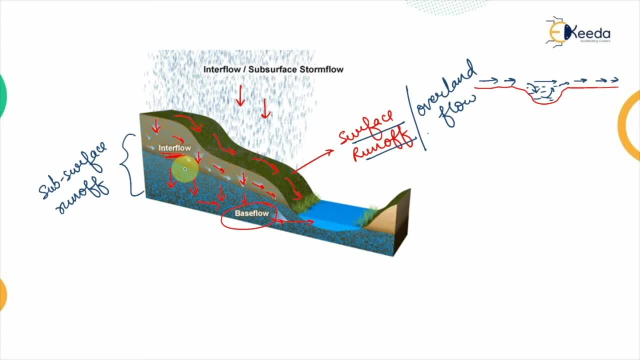 That infiltrates and moves laterally, That means horizontally, within the upper crust. So this interflow, That is within the upper crust of the earth surface And it returns to the earth surface At some location Away from the point of entry. 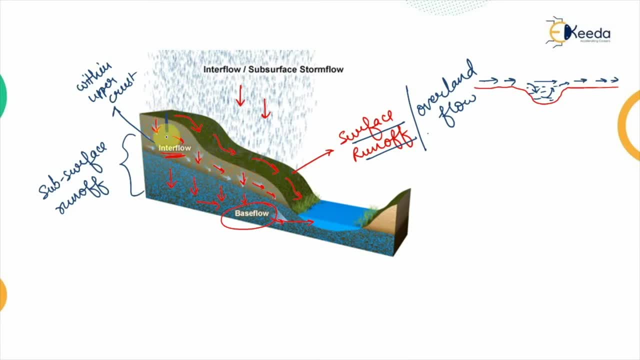 So if a certain drop of water, If it has entered through this point, So after flowing horizontally It will be coming out here. So that is certain other location Or certain distance away from the point of entry, This component of the runoff. 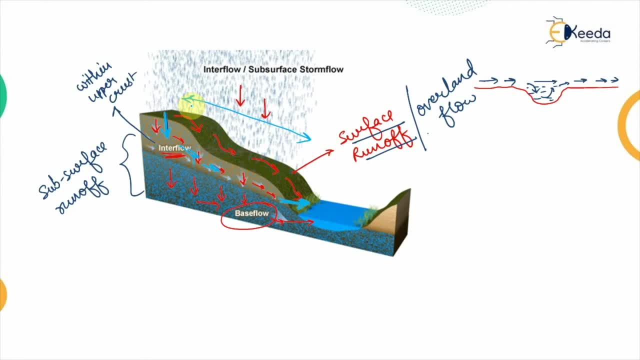 Is known as the prompt interflow, Or the seepage, Or the quick flow, Or the quick return flow. Now, that depends upon the geological condition, Whether this upper crust is permeable or not, And what is the composition of this soil. 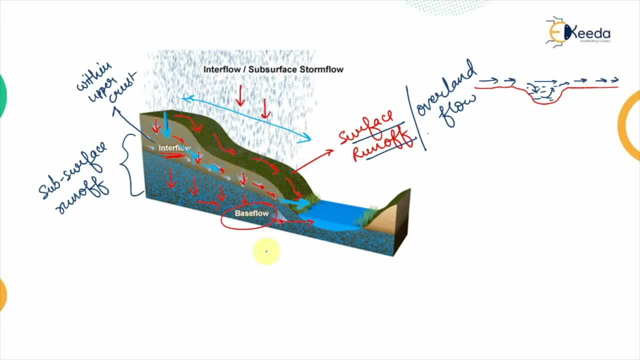 There are number of factors on which it depends. The second component of the subsurface runoff Is known as the delayed flow, Or that is also known as the base flow. Now, when the water is seeping down to the greater depths, What is happening? 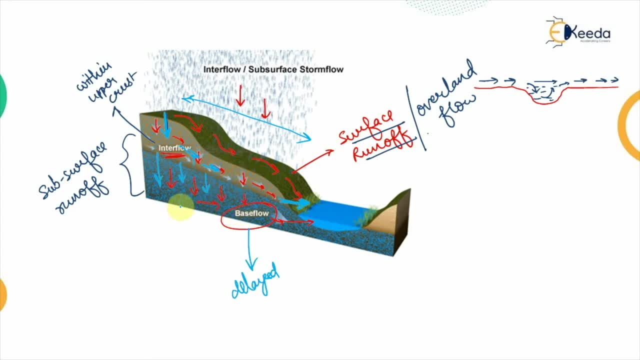 This water is not able to apply The required pressure So that it can come out. So when it is having the suitable depressions along with it, Along the level of its flow, Only then it will be coming out naturally. Otherwise, this water, which is flowing below the earth surface, 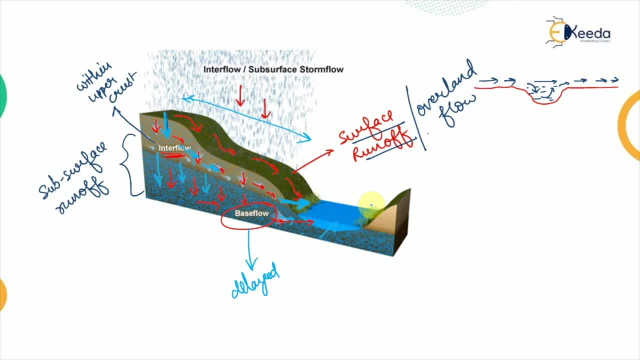 At the greater depths That return to the surface After a long period of time. And when we are saying a long period of time, We are meaning by months or the years, And that is why this is known as the delayed flow, And since it is flowing below the ground level, 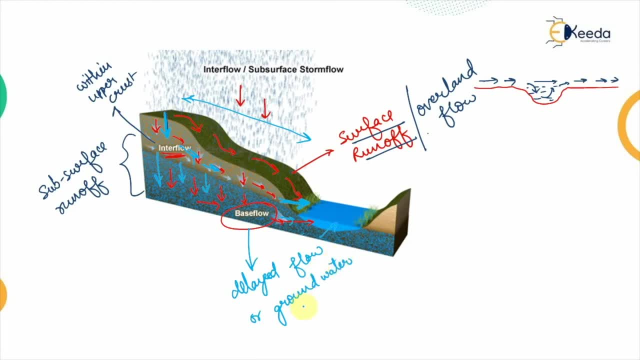 That is why it is also known as the ground water runoff, Or the base flow. Now, when the perennial river, In case of the perennial river, Which flows throughout the year, This component of the base flow, It represents the dry weather flow. 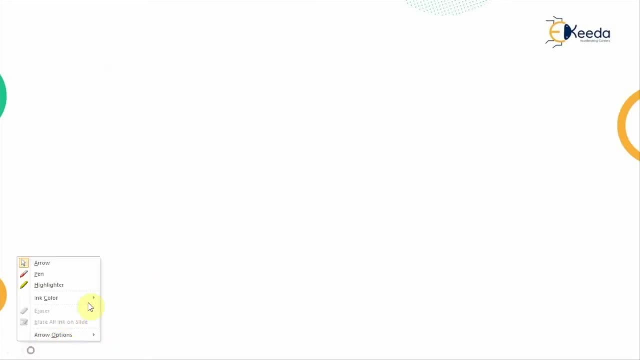 Now there is one more classification of the runoff That depends upon the time delay between the precipitation and the runoff. So, depending upon the time delay between the precipitation And the runoff, So let's say, if the precipitation is happening on Sunday. 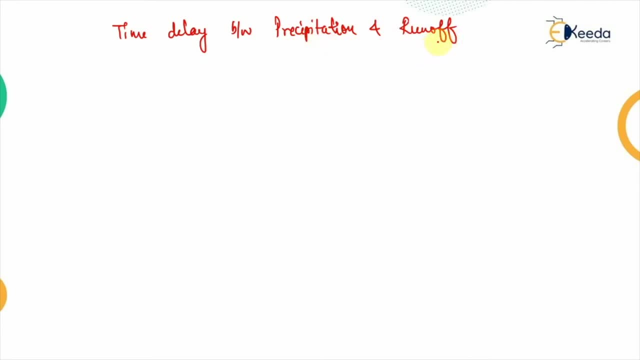 And runoff is being collected on the Monday morning. So that means there is certain difference between the precipitation and the runoff. So that is also one factor Based upon which we classify the runoff As the direct runoff And the second one 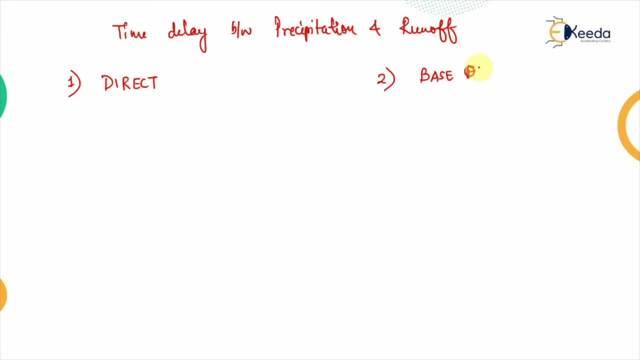 Is known as the base flow, So the portion of the runoff Which enters into the stream immediately after the rainfall. So this is the component Which is entering the streams immediately, That is, the direct runoff. Now this involves the component. 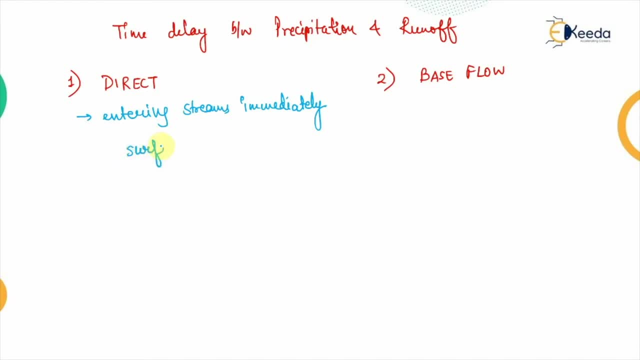 Of the surface runoff, Because that is joining the stream directly, And the second component is the prompt interflow, Which is the water which is flowing below the earth crust Or within the upper crust of the earth surface. These two components enter the stream immediately after the precipitation. 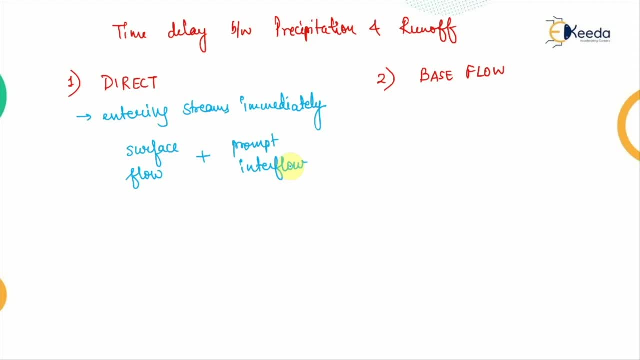 Now, the volume corresponding to this Is known as the direct runoff volume, And the discharge corresponding to it Is known as the direct runoff discharge, And the representation of this runoff Is done in the form of a plot That is known as the direct runoff hydrograph. 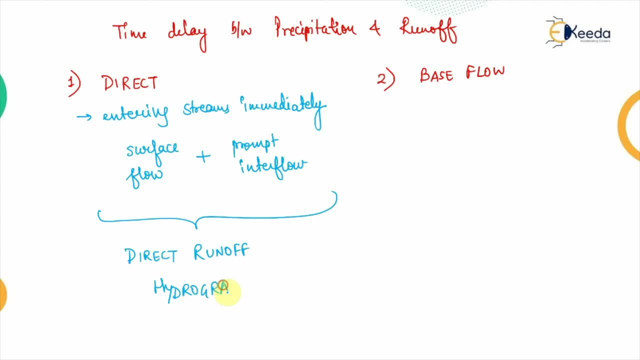 And these hydrograph Are basically the representation of the runoff against time. So only one component is left, That is, the delayed flow, And this delayed flow is known as the base flow. So volume corresponding to this, That will be known as the base flow. 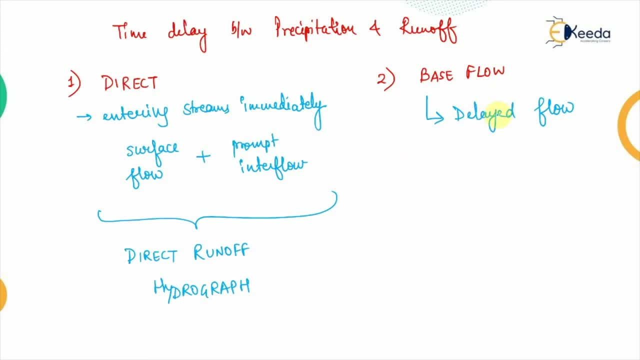 Or the flood runoff volume, This base flow that is also known as the Flood flow, And therefore this Will be represented In the form of the Flood runoff Hydrograph. So these are the another type of Distinction between the different type of runoffs. 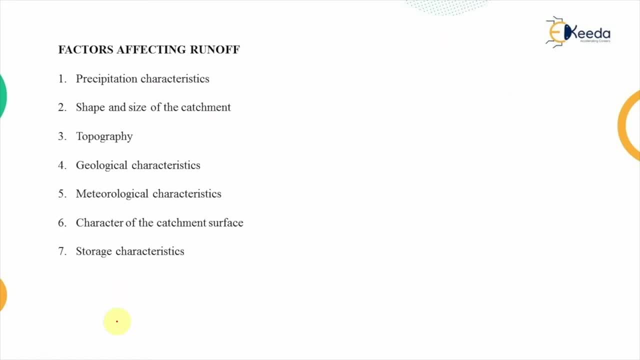 Now, this runoff depends upon the number of factors. So what are the factors which affect the runoff? So, first one is the precipitation characteristics. Now, what is this precipitation characteristic? It is the most important factor for the runoff. So if the storm is heavier, 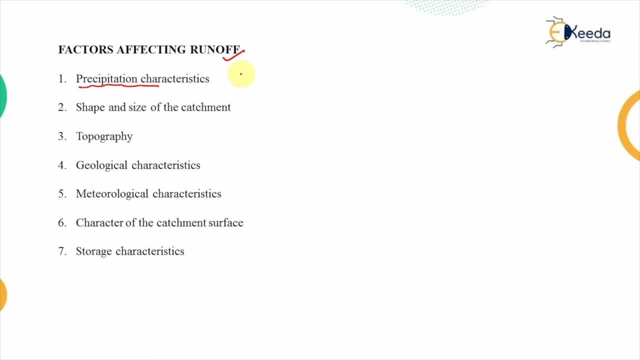 So, and if it is for higher duration, That obviously it will be having higher runoff. If, within an area, More rainfall is occurring, Obviously the precipitation that will also be higher. But if the rainfall is very less Over the area, Then the precipitation 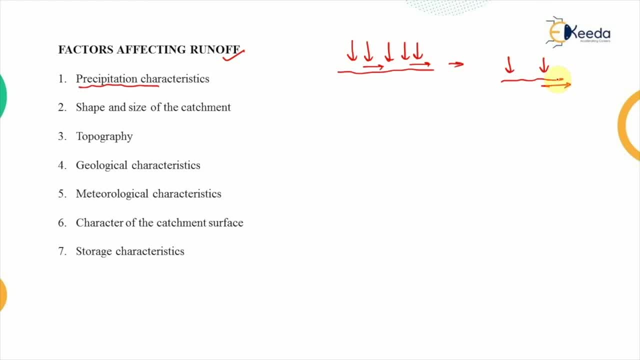 Is lesser than the runoff will obviously will be lesser. So there is a direct relationship between the precipitation and the runoff. Then the second of the factor that is known as the shape and size of the catchment. So if the size of the catchment 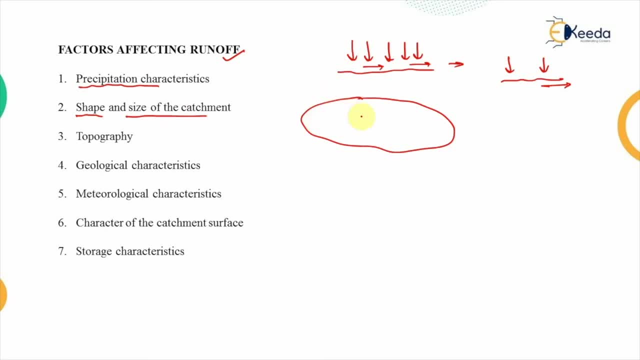 If that is very large Within this catchment area, If we compare this to another catchment Which is having the lesser area, In both the areas We are having the same amount of the rainfall, So obviously the runoff will be higher. 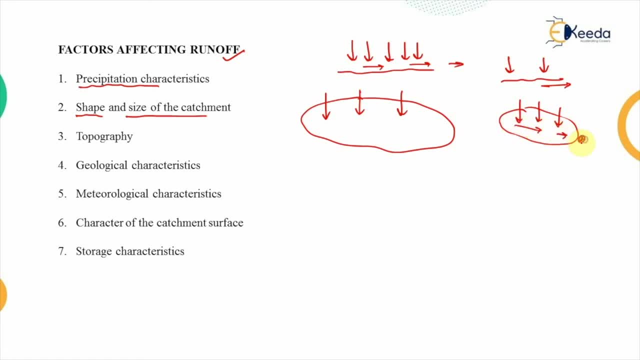 In case of the second one, Because it will be reaching the outlet point. This point is known as the outlet point At which the water is collected. So the water will be reaching the outlet point In the second case Earlier than the first case. 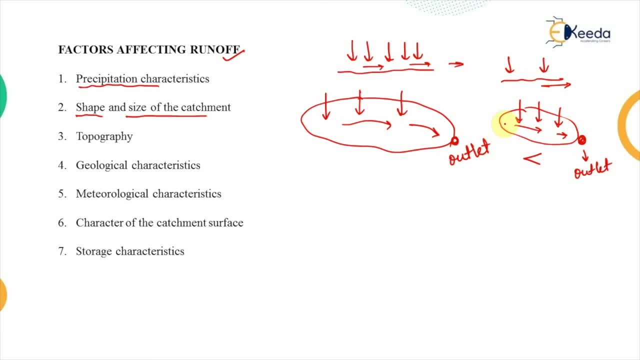 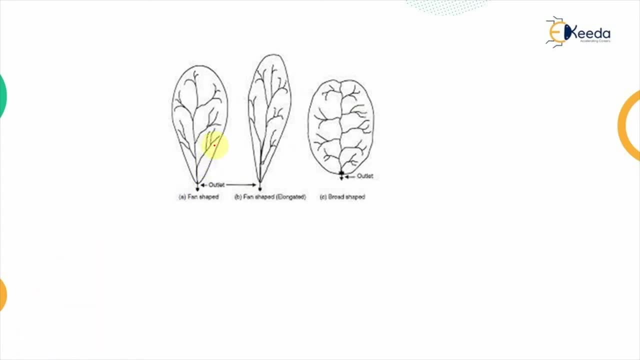 And that's why the size of the catchment matters. Now, what is the factor of the shape? Now, depending upon the different shapes of the catchment, The runoff is different. So, for example, This is known as the fan shaped catchment. 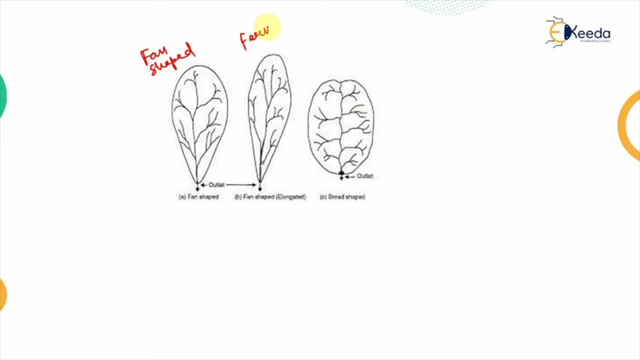 The second one is known as the fern shaped catchment. The third one is known as the broad shaped catchment. Now, these are the outlet points Of all the three types of the catchments. Now, if we are having the rainfall here, 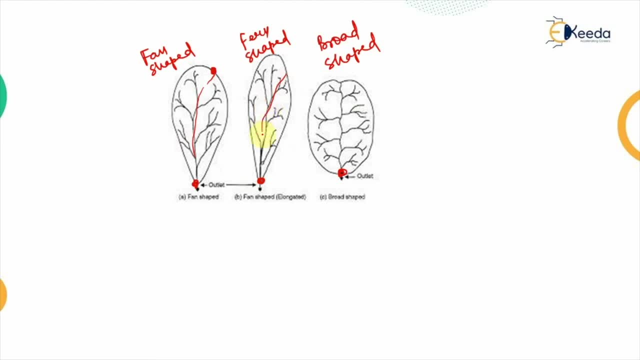 So the rainfall will be reaching the outlet point Earliest in case of the fern shaped catchment area, Then the second quickest. It will be within the fan shaped area And it will be last in the broad shaped area. That is the impact of the different shapes of the catchment. 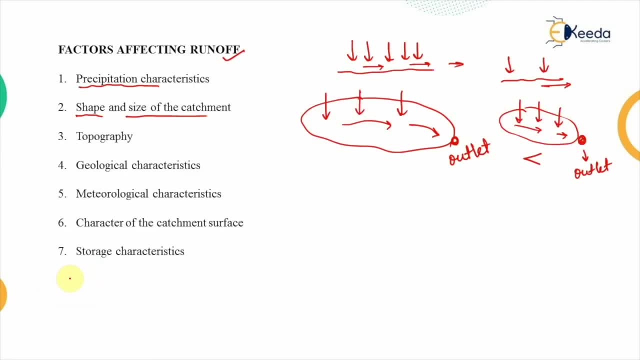 Then what is the impact of the topography of the catchment? So this runoff, it depends upon the surface smoothness and the slope. So if the slope is very steep, So the runoff will be happening very quickly. If the slope is flat, 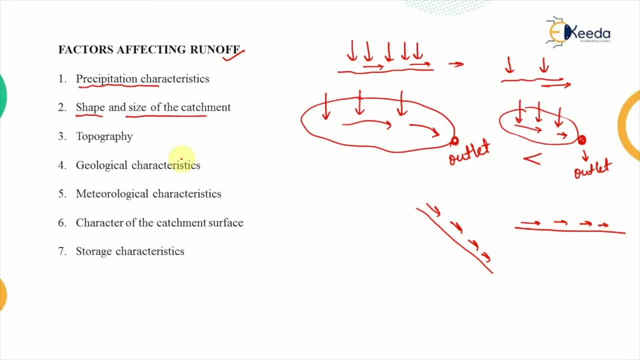 Then this runoff will be happening very slowly. So that is the impact of the topography of the area. Now the next one is the geological characteristics. Now, within this geological characteristics, The most important one is the permeability of the soil. 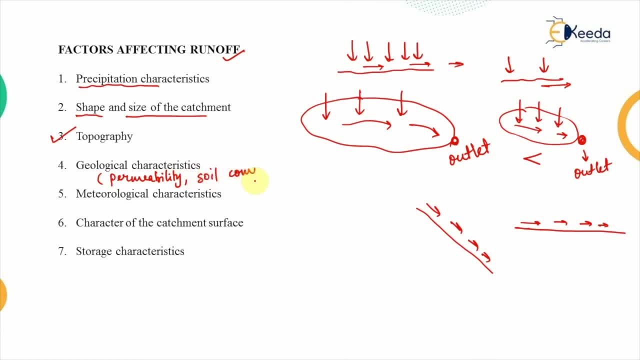 And the soil composition. So if the permeability of the soil, If that is very high, Then the seepage that will be happening, That will be also very high, Increasing the components of the subsurface runoff And the surface runoff will be lesser. 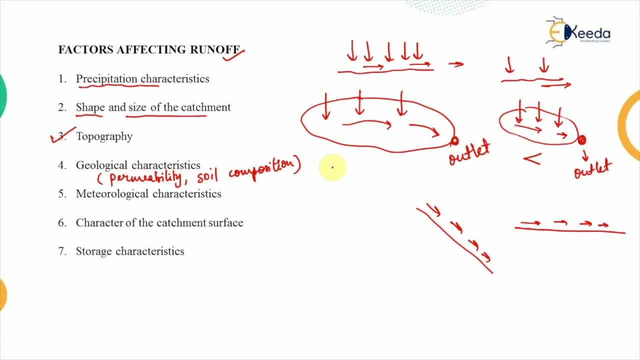 And if the surface is rocky, Then the absorption will be almost nil. That means resulting in the more runoff. So that is the impact of the geological characteristics. Then the next one is the meteorological characteristics, For example The temperature, The wind conditions. 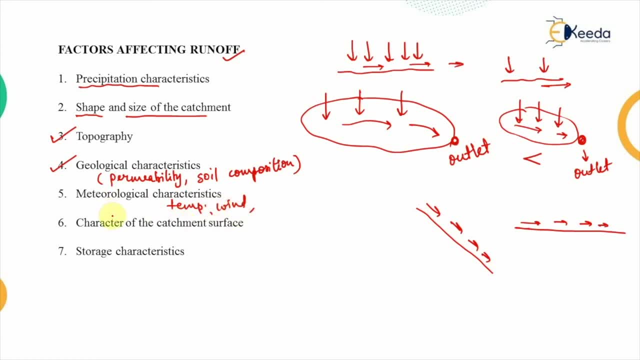 Or the humidity. All of these fall under the meteorological characteristics, So if the temperature is low, That means there will be lesser chances of the evaporation. Therefore the runoff will be greater If the temperature is high And the greater wind velocity. 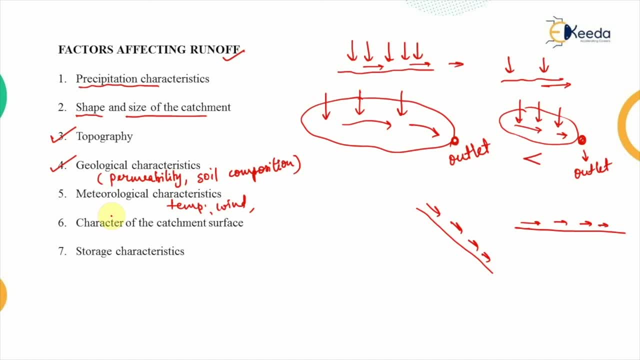 That means there are more chances of the evaporation loss And because of that there will be lesser runoff. Then the next factor Is the character of the catchment surface. So if the catchment surface is drained or unbrained, That decides whether the runoff will be very quick or will be very slow. 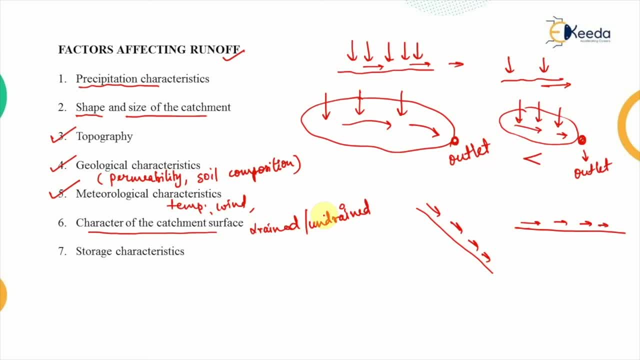 So if there are no natural drainage, Then the absorption losses will be more And because of that That area will be having lesser runoff. For example, If you are having certain vegetation in the area, Let's say this is the area.